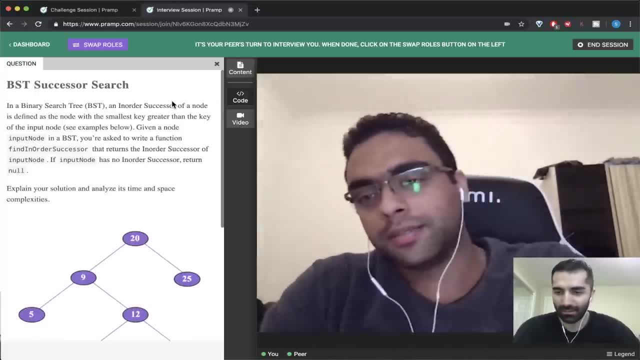 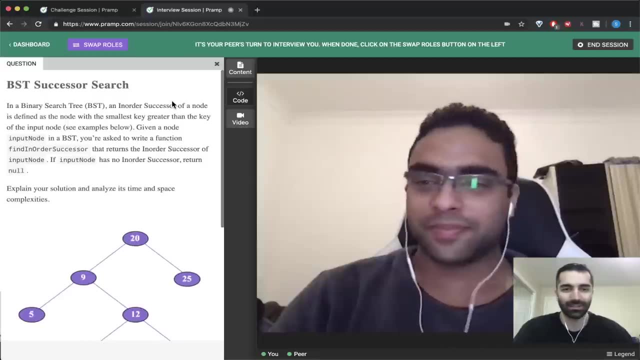 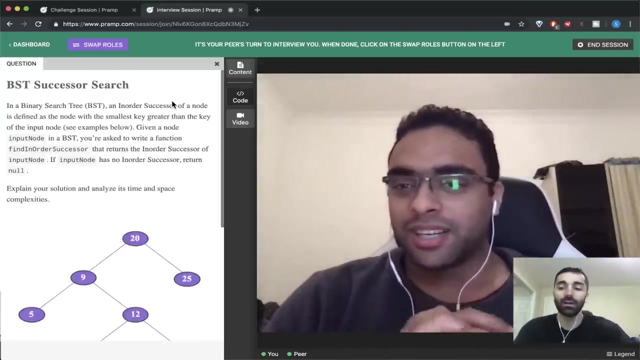 Hello, Hello, are you hearing me? Yeah, I can hear you. Can you hear me? Yeah, I'm hearing you. fine, Great, How are you? Pretty good, I'm pretty good. I actually just found out that as a video interview. So, yeah, okay, It's okay. Yeah, Is this your first time using this platform? No, I'm just before, but from two or three months ago, So recently. Yeah, I've used. I've used other ones, But this is my first time using this particular one. Okay, Yeah, Okay. 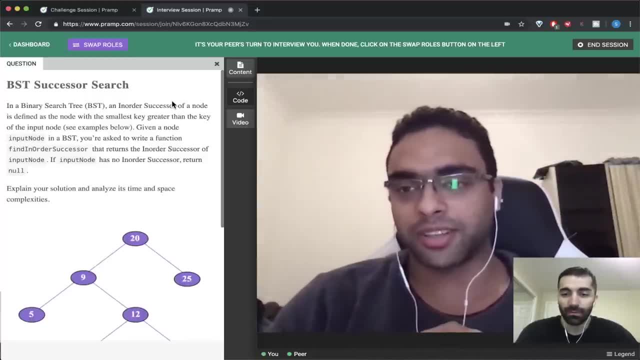 Are you already software engineer or you're seeking for a new opportunity? I'm looking for new opportunity. Yeah, Yeah, What about you? I'm working recently in Bloomberg London office. Okay, Yeah, Okay Yeah, I'm in Bay Area, California. 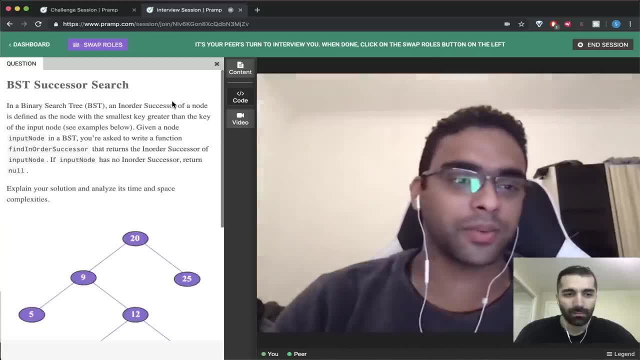 Okay, Yeah, Okay, Cool, Nice to meet you, So it's supposed that I will start asking you first, Okay, So, as you see, you want some time to read the question for it. Um, yeah, let me see. Okay, so it's the BST successor search. Yeah, Okay. 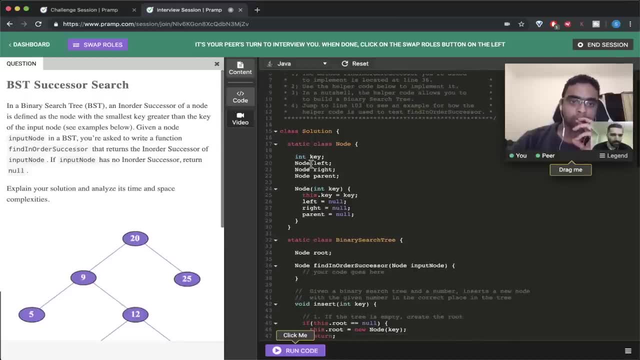 Okay, so in a binary search tree, an in order successor of a node is defined as the node with the smallest key greater than the key of the input node Given a node. yeah, binary search tree, you're asked to write a function, find in order successor- that returns the in order successor of input node If it has no in order successor return null. 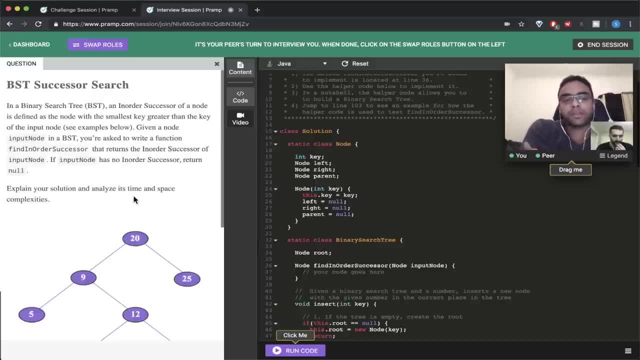 Yes, So what? what you need to do? given a node, you have to get the smallest node which have a smallest value greater than the given one, If it exists. if it doesn't exist, just return null. Okay, And in the existing code you have the. 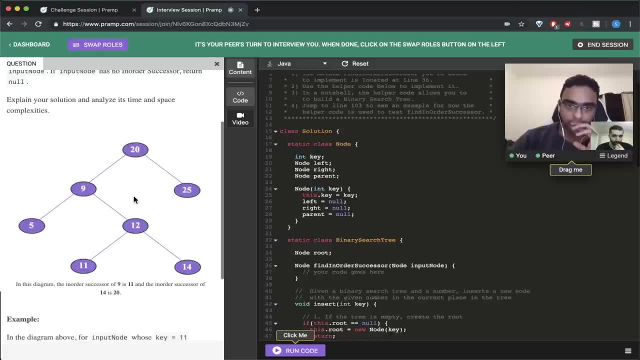 the struct for the node, which you will code in Java. Yeah, I'm going to code in Java. Okay, So in you have a class for node that contains the key and lift Android and you have access to the parent itself And the constructor takes a value for the key. 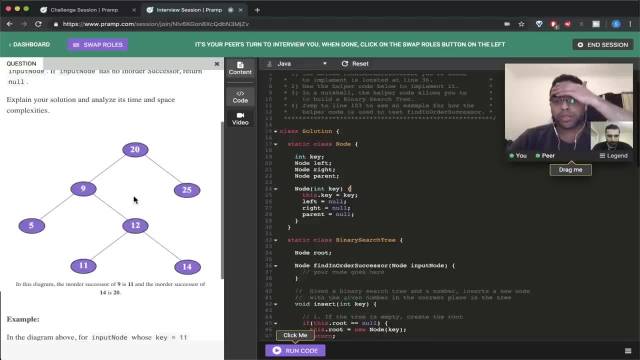 And for the method which we need to fill, which is: find in order successor, take the input node and return a node which is a target one and null it if it doesn't exist. And you have the, you have some logic for the insert, but you don't need to take care about that. 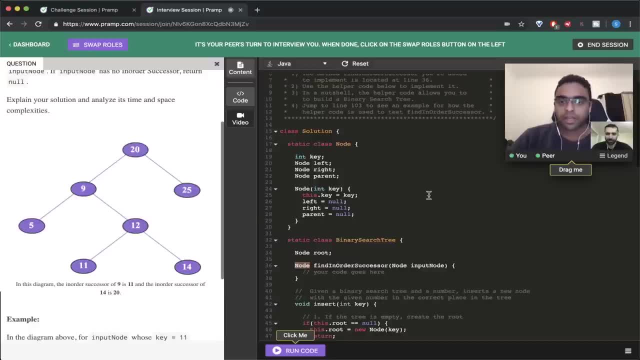 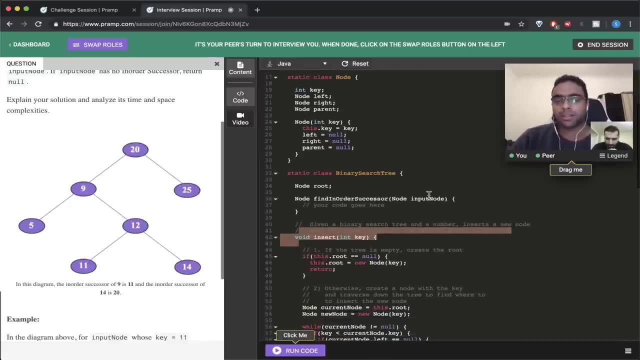 Okay, I'm sorry. can you say that last part again? You don't need to take care about the logic for the insert method, Which is this part. Okay, the insert method. Yeah, it doesn't matter for you. Okay. 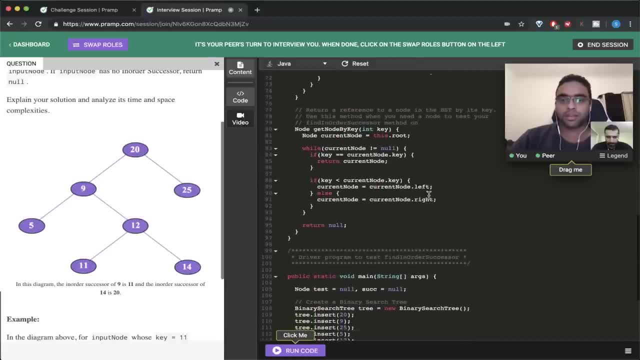 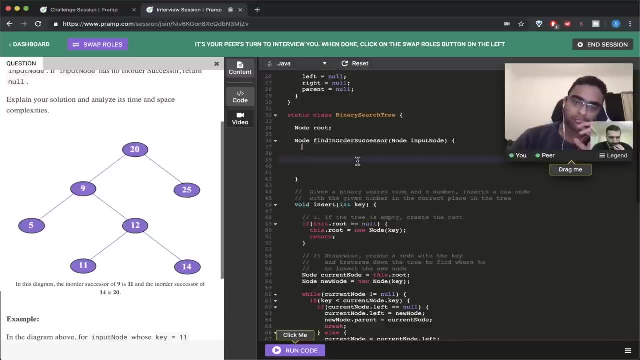 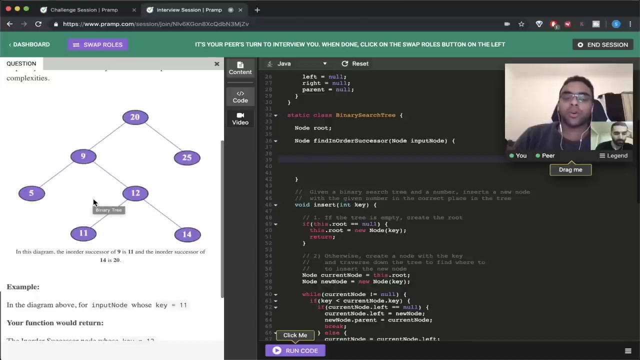 You will not. you will not need something like that. So all you need just editing, Write your code here in this part Or this problem, Okay, And then so the input isn't the necessary, the root: it can be any node in the tree. copy any of something like the tree example on the list. Okay, Yeah, I given you something like nine. Okay, So I'm searching for the node which contains the element greater than nine and the same time is the smallest one, So it will be 11.. Right, 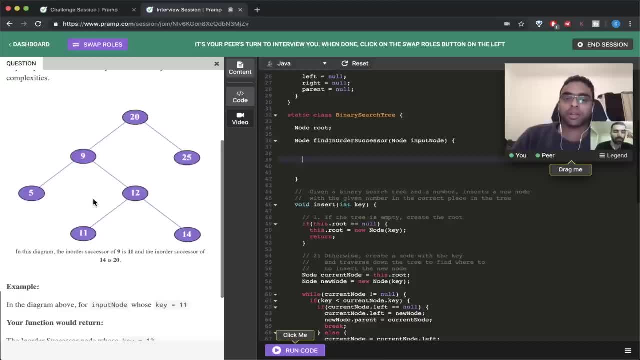 Okay, So I'm expecting when I give you nine as an input. you got me the note, which is 11.. This one Something different. If I go, if I gave you 14, you need to return the root, which is 20.. 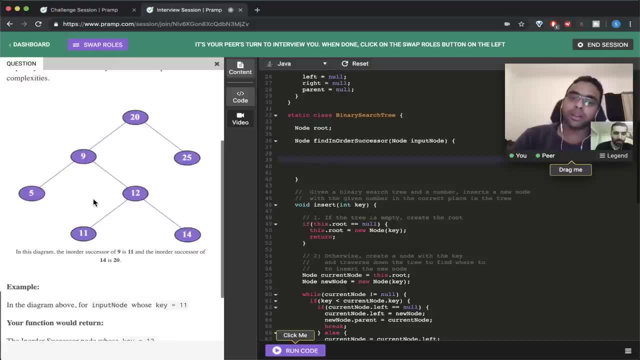 Okay, Because it's the first node greater than 14.. I see, Okay. So if I do have a nine, I want to return 11.. Yes, if I have a 12,, I want to return 14.. Yes, right. 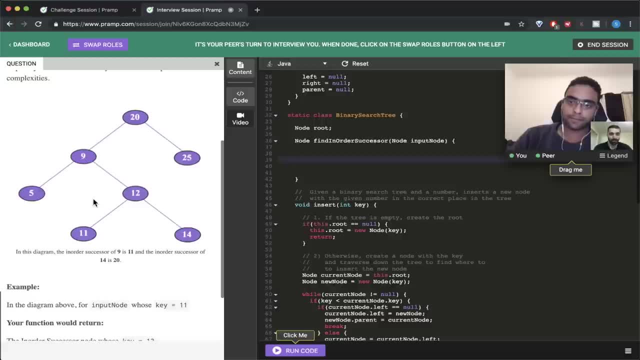 Okay, And I do have access to the parent nodes. Exactly, You have access to the bit there. Okay, So just get going over a couple examples. Say you give me 1111.. Yeah, then the in order would be 12.. Right, Exactly, Okay. 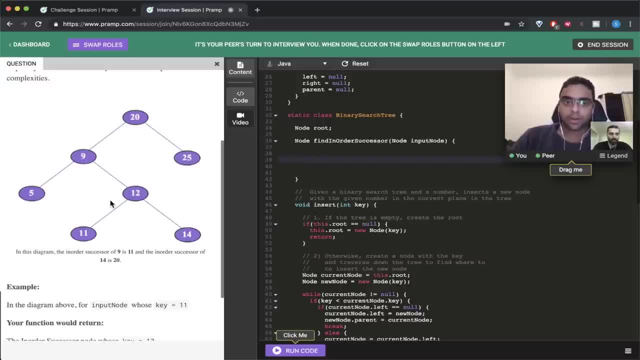 So I'm just trying to think of the different cases that we can have Here. Okay, So, yeah, let's, let's just say, use 12.. As an example would be four. So So, if so, if we're using 12, and we're going down the tree, it has to be on the right side. 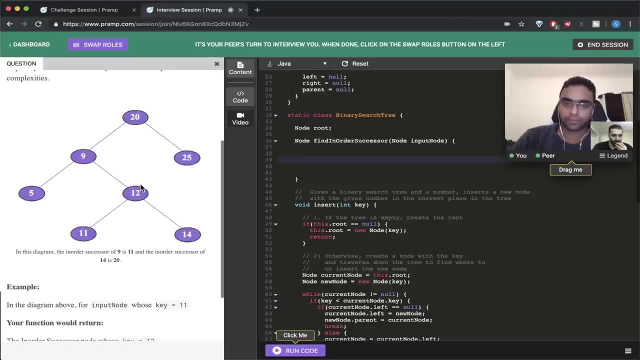 Okay, But think about it: if I give you nine and there's no 14 there, Yeah, Yeah, if you give me 12, and there's no 14. Then the answer would be 20.. Right, If I give you 12?. 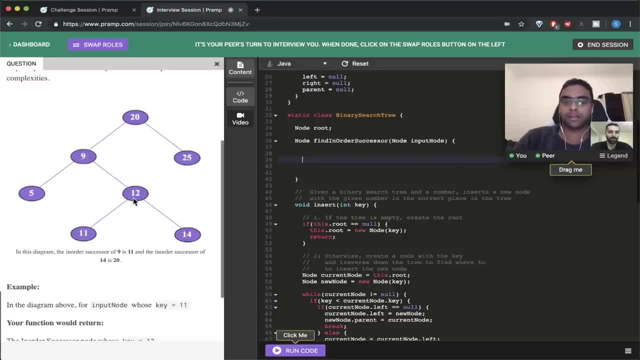 Yeah, if you give me 12, and there's no 14.. Yeah, if that didn't exist, then I would have to go up. Exactly, Yeah, I would have to go up And then I would have to go. 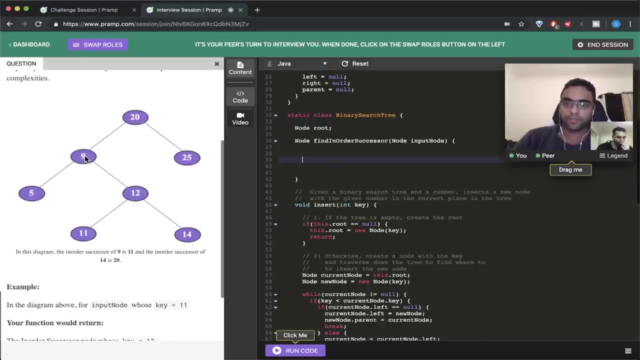 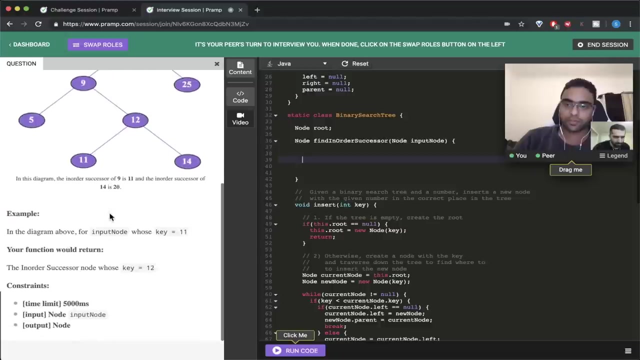 I would have to check which side I'm coming from. Yes, And if I'm coming up from the right side, then I would have to go up again. Yes, And then that would be the answer. Okay, It just seems like there's like a lot of different cases that we could have. 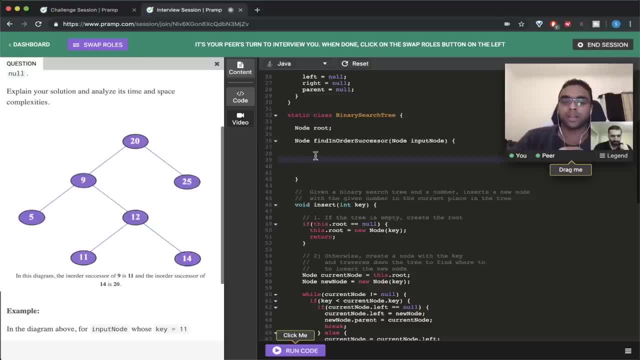 I think, I think we have two cases Right And you said, you said it correctly. First case which, if I give you nine, I'm expecting you to return 11, which seems that I will go down right, Right. 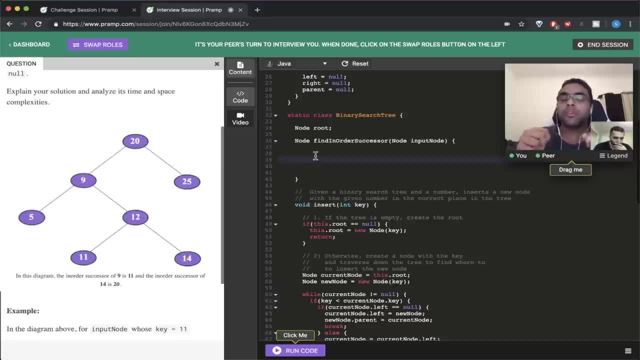 But in the other case, if I give you 12, without having 14, I need to return 20, which I need to go up, Right. So think about it when I need to go down and when I need to go. 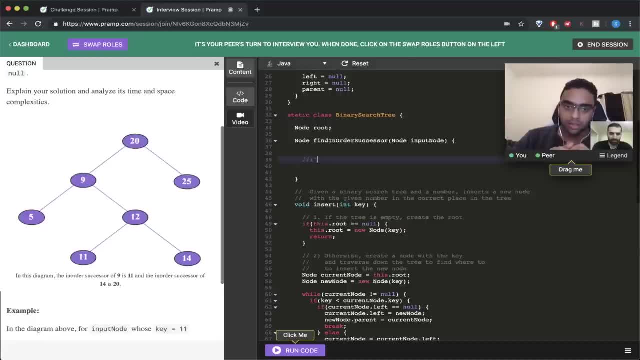 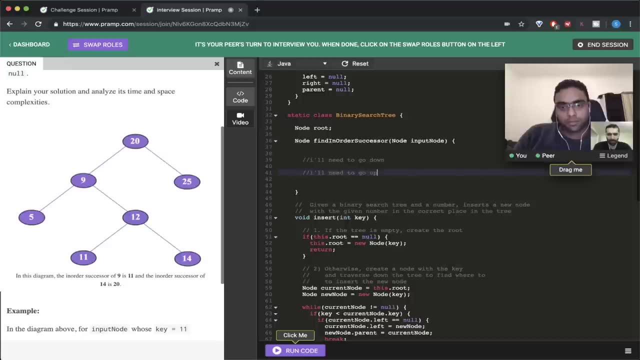 So you have: yeah, I'll need to go down case one, And then other cases I'll need to go up, Exactly. So let's start with going down. Yeah, When I need to go down, Okay, yeah, if you need to go down, then you want to always go. you want to check if there's a right node. 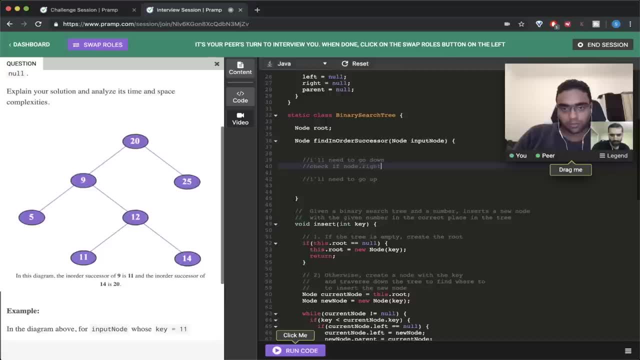 Check if node dot right exists. Okay, If it does exist. If it does exist, then yeah, you want to go down and then go all the way to the left. If it exists, right, So think about it. If I give you 12, without having 14, this is the same right. 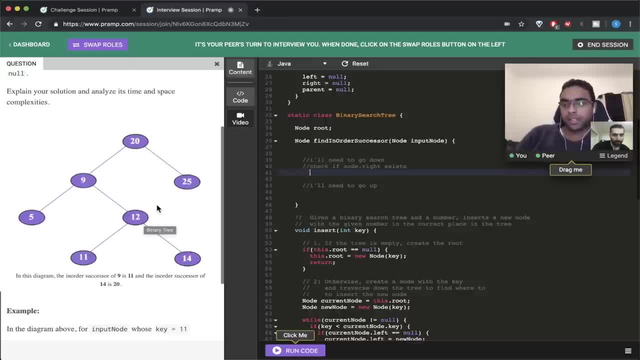 I give you a node which doesn't have a right child, so you need to go up, not down, not down. right, Right, right. So if you don't have a right node, you need to switch to the second case, which is: I will. I will need to go up. 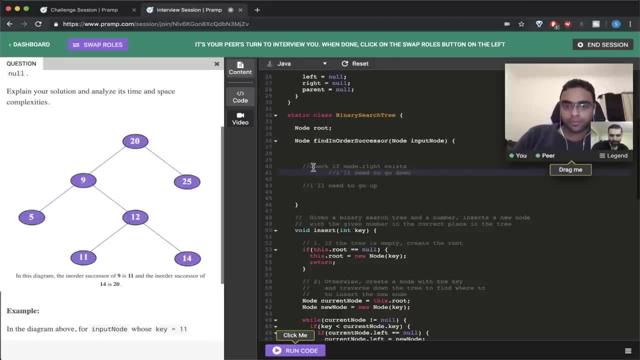 Well, maybe I'll do so. so the first case will be: if right node exists, go down to the to the right. Okay, Go down. And now let us think about something else. If I gave you nine right, 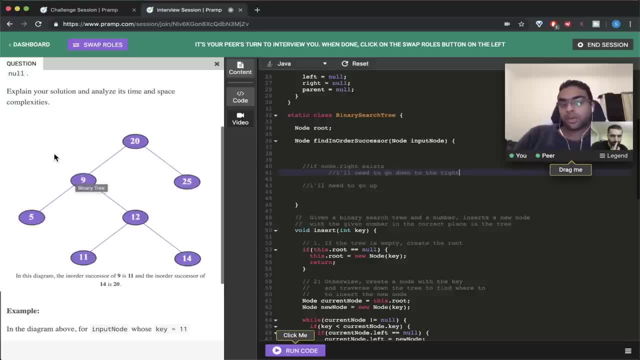 Yeah, And you have a right node, which is 12, which node you need to return. You need to return 11.. Right, Yeah, So you go down to the right And then At this point- Yeah, At this point- check if uh left exists, and then, if it does, I believe, then you just want to go all the way. 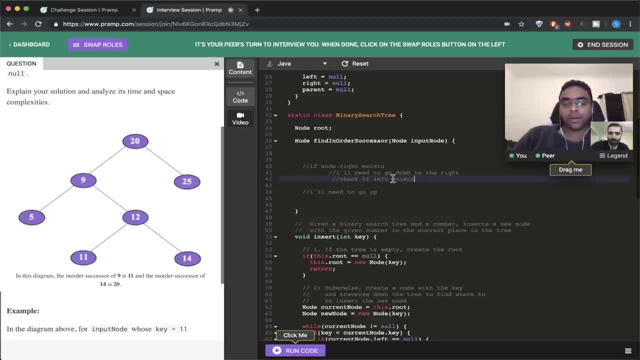 You want to keep going to the left until you get to a null node, Okay, And if it doesn't exist? if it doesn't exist, which means, if I give you nine, yeah, To turn 12 without having 11, right. 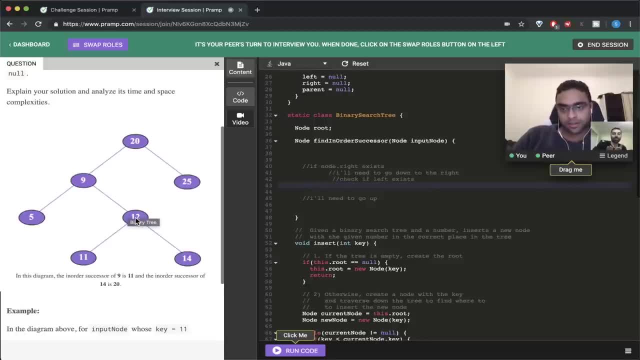 Right, Right, Yeah. So if it does so, cause basically you're just go, you are still, you're going to the right and then you are still going to the left until nothing exists. So yeah, if there's no 11, then you would just, if you had like a loop, it would just stop there. 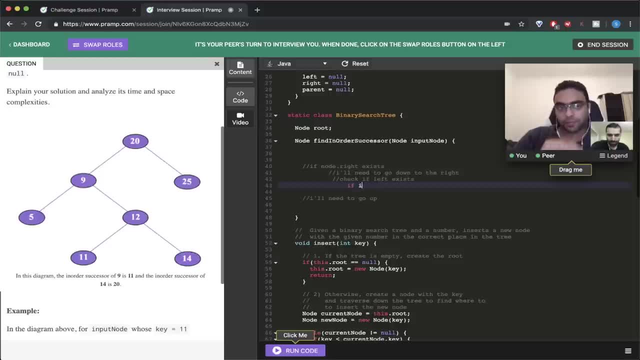 Exactly, Uh, okay, So, uh, if it, if it exists, go all the way left until no, And I think that's, and then you should be done at that point for this choice. So I think once you do that, then you're done. 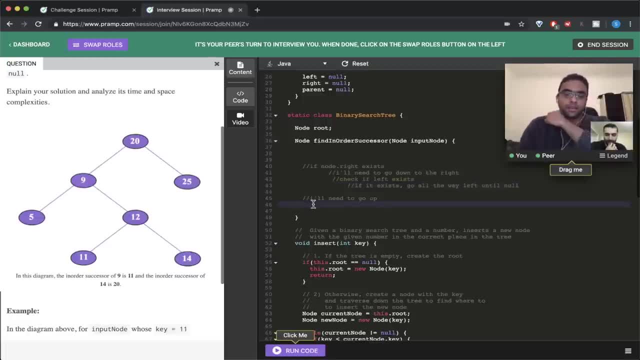 Uh, yeah, This, yeah, I think, yeah in this case, Yeah, Okay. So then the other case, when you need to go up, yeah, Um, so let's think about if I give you 12 without having 14, yeah, then you would have to go up. 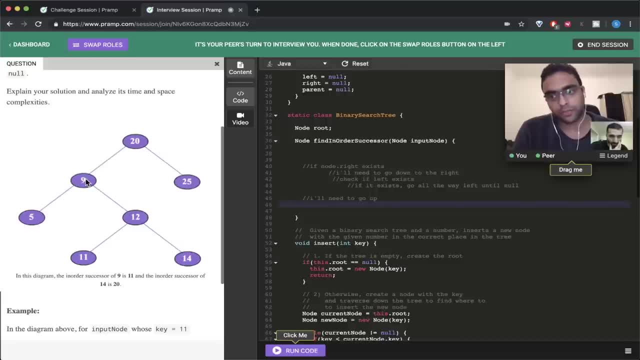 Yeah, Tell what you have to go up, and then you'd have to go up again. So you have to go up, and then you have to go up again until you get to 20.. Yes, So when you're going up, I think you want, you need to check which side you're coming up from. 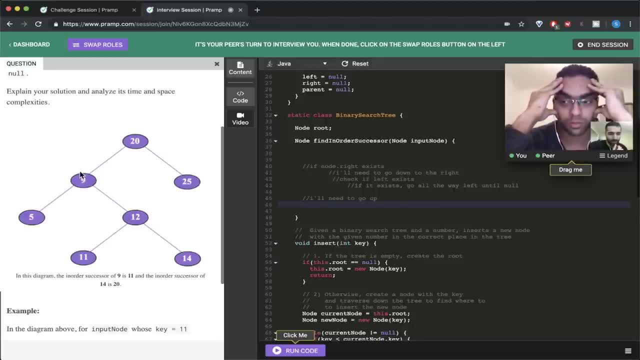 So if you're at nine, once you go up you'll say: if nine dot right equals the node that we're on, Then you go up again. Mm-hmm. But let's say we're on a, we're on 14.. 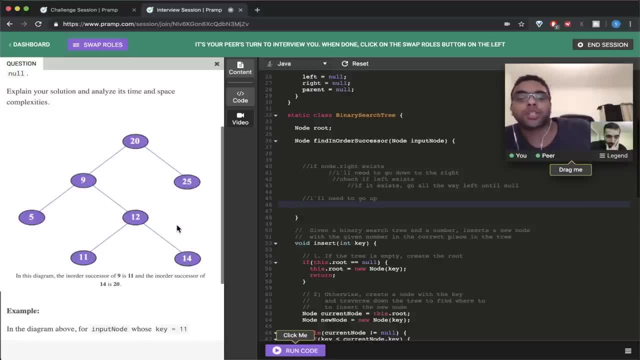 Yeah, I agree with you If I give you 14, so you will check. you will check that you don't have a right right child. So you decide you will go up. So you will start with 12 and you are coming from the right. 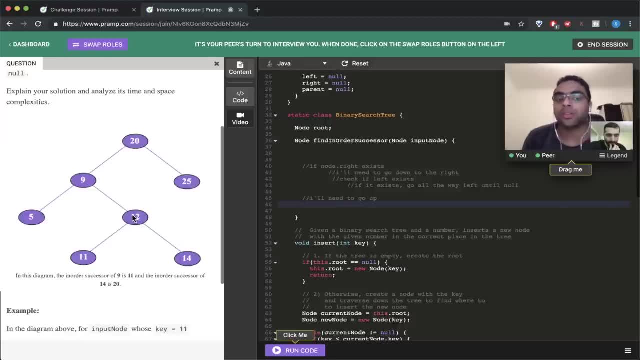 So it seems that you need to continue, right. Yeah, You need to continue. So you will continue: 10,, 10,, 9.. Right, And you are coming from 12, which is from the right, Right, So it seems that you need also to continue, right. 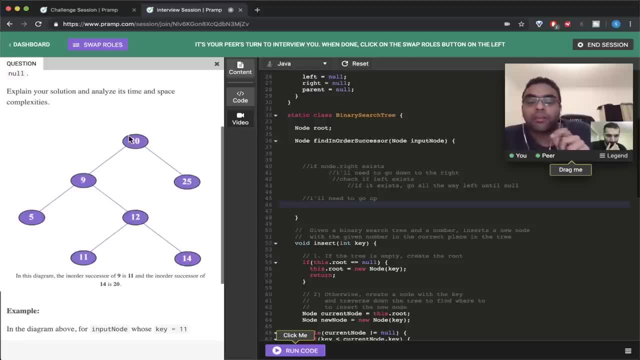 Right, You need to go up again. So you will go up to 20 and you are coming from left this time, Then, So you need to stop and you need to return 20,. right, Right, right, right, So okay. 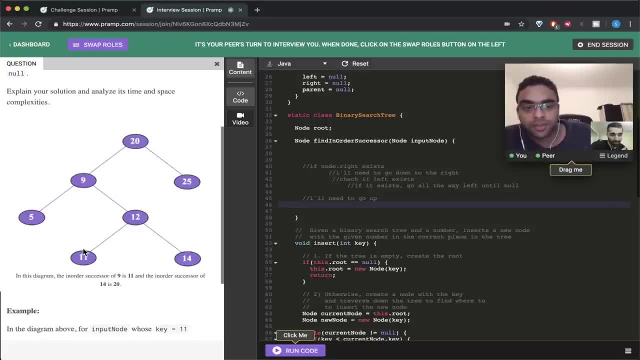 So in this case, if you're coming from 11, you're again. you see there's no right node. Yes, So then you go up to 12.. Yeah, Yeah, You check that you came from the left, So you know you're done. 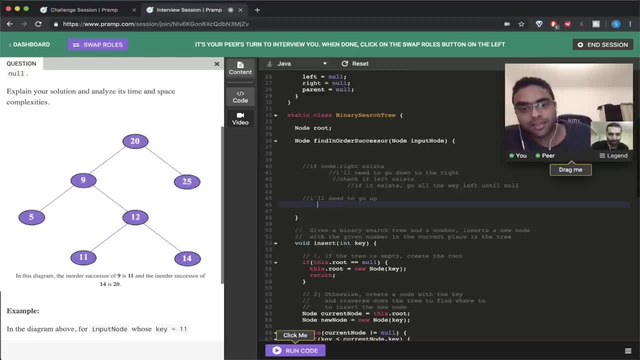 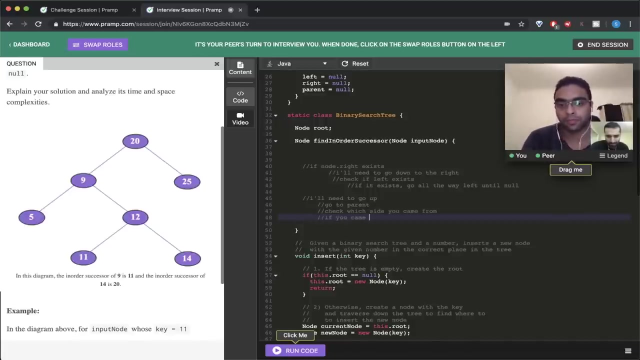 Exactly Okay. Let me write that down. Okay, So, if you're yeah, So if you're not coming from the right, then you want to go to parent Check which side you came from. Exactly Okay, So if you came from left side. 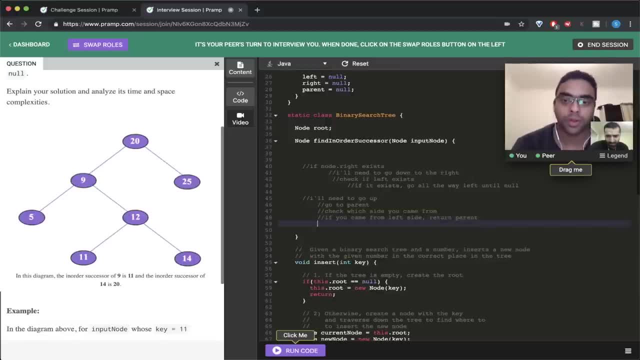 Okay, Okay, Okay. So if you came from the right side, you want to return the parent? Okay, If you came from right side, go up again, Okay. And then you always have the case where if you, if you are at a say, you're at the root. 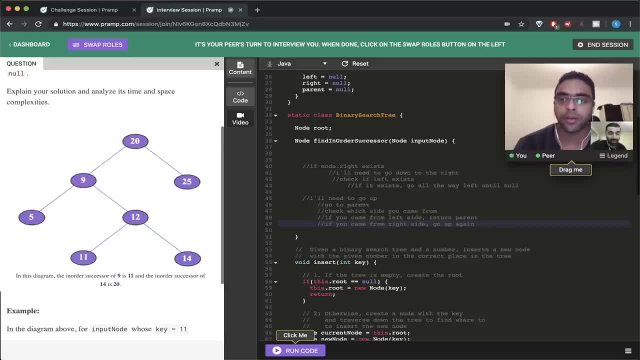 and there is no parent. Okay, Then This will be covered, right, Because if I give you 20, first check, well, well check if I have a right child which is a 25.. Okay, So I will return it, right. 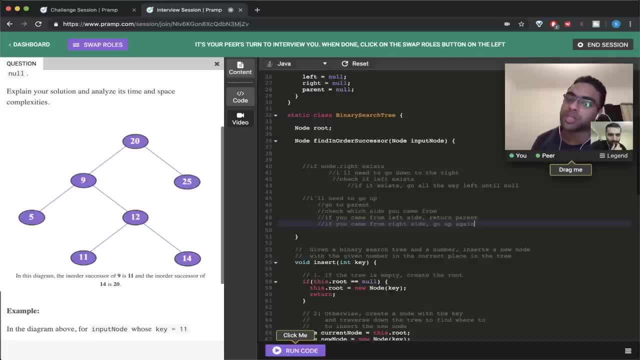 But if I don't have 25, I would go to the second check, which is I will try to get my parent, which I would find that I don't have any parent. So I can return 20 directly, Right, Right. 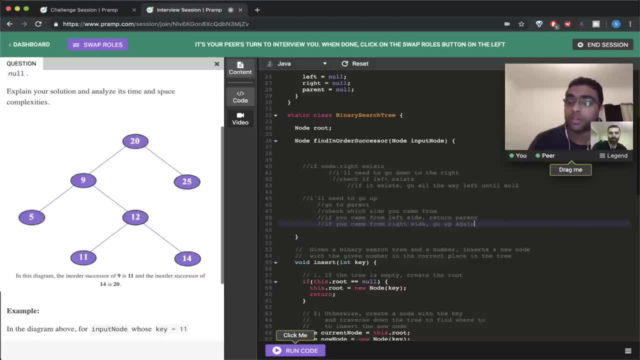 But I think you'd have to check for that. Yeah, Yeah, You'd have to do some kind of check to check your parent. I think it will be included. It will be included in the checks. a check, which is you will do it here. 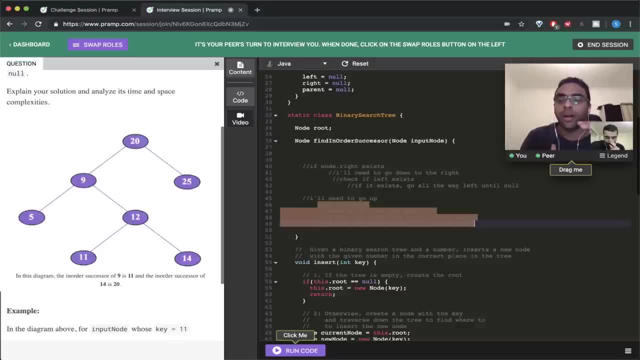 Right, Because this part you will add, you will do this part in while loop, right? And every time I'm going to check the parent If the parent is null, so you need to stop right now, Right, Right, Let's do some coding. 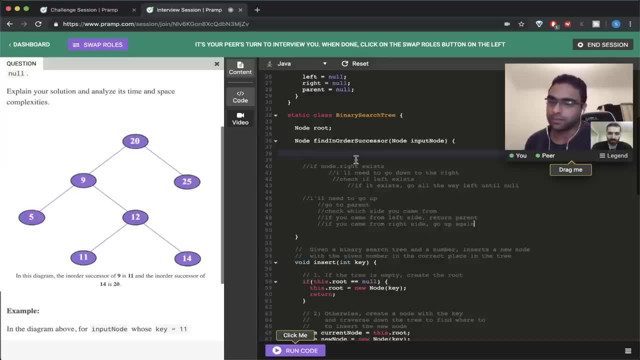 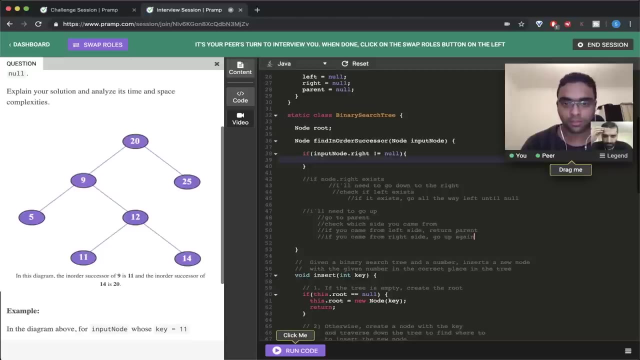 Okay, Um, so we are. we're given input node, We'll say: if input node, so if input node, uh, yeah, it does not equal. no, then, Um, maybe we'll do a recursive call where again, we're just calling this on. you will solve it in recursive. 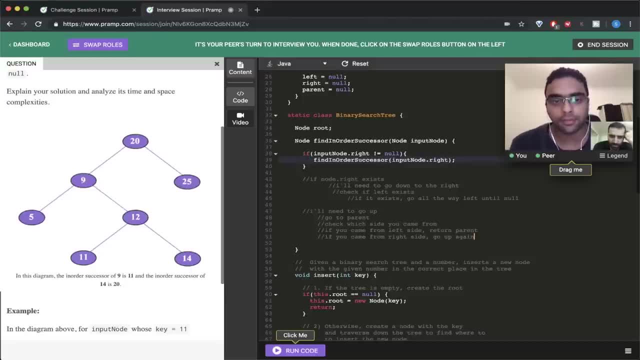 Okay, Yeah, Um, I mean, we could use pointers as well and just have them go up and down. Um, yeah, you can just update, but okay, If you prefer recursive, just go ahead. Yeah, Okay, So yeah. 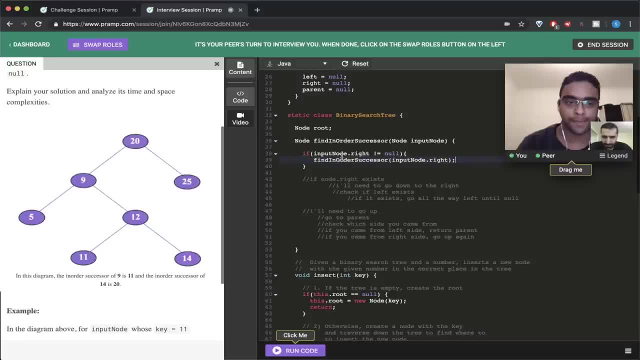 So if, like we said, if right exists, actually it might be easier to do it, Let's just, yeah, let's just do this. Um so, input: right Does not equal No, we want to call it. 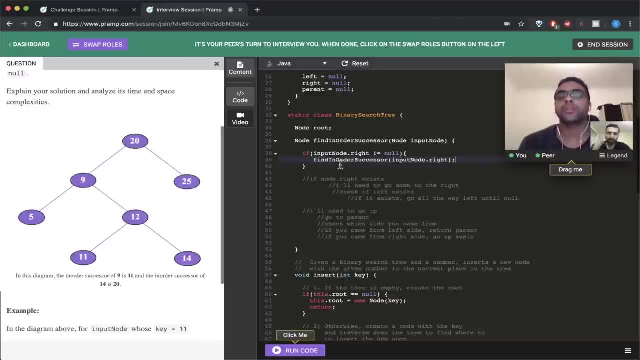 You can, you can't, you can't recursive on the same method because if, if, if the node to the right is exist, right, You need to use some different logic, which is, You need to get the most left node right. 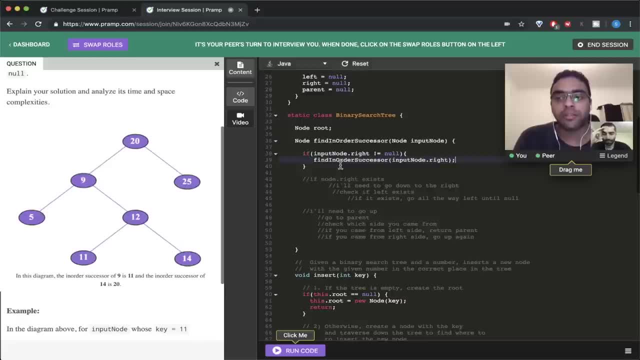 So you need to write a separate method which can, given a note, get the most left, one Right. So I think, I think you need, you need to go here, right here, and just type a method which is get most left. 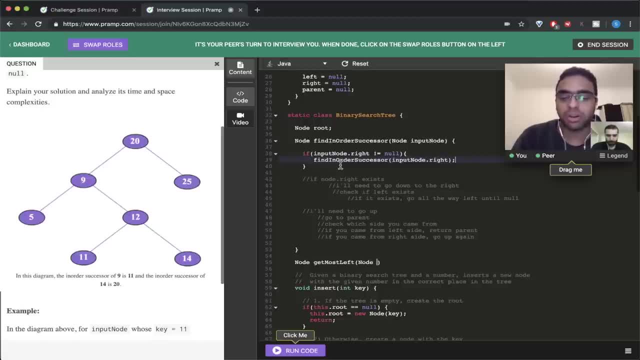 Right, And you can give it a note which is: call it X, anything, Okay, And it's not responsible for getting the most left child Right, right. So yeah, you'll just write um. if X dot left is not yeah, if it equals uh, no, then you'll just uh: return X. 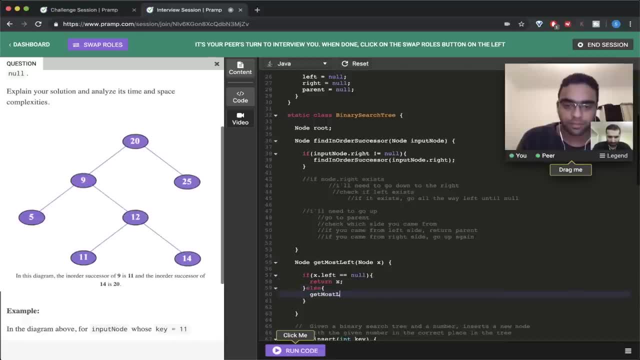 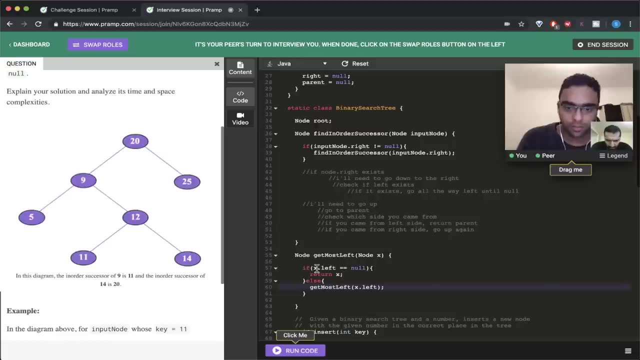 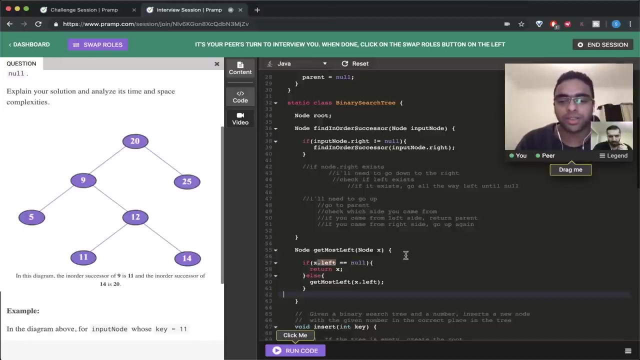 Uh, otherwise uh get most left, uh, X dot left. But uh, this, this check should be like that: Okay, Okay, X. and well, here now, you, you, you can't do that, because if you don't, X, okay. 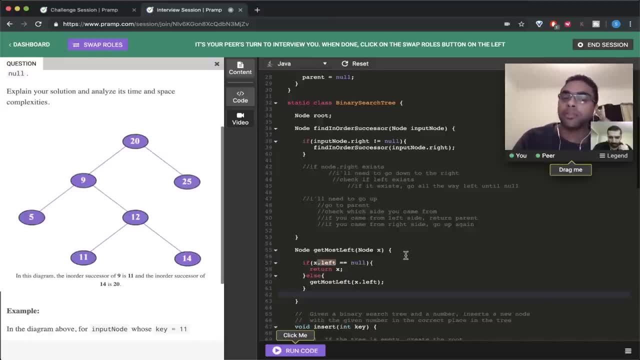 Let's assume that you you will start with I gave you, I gave you nine. Okay, So you will. you will pass to this node, the node 12, right, And you will start out trading. So the first time you'll check is: 12 dot left, equal, equal, none. 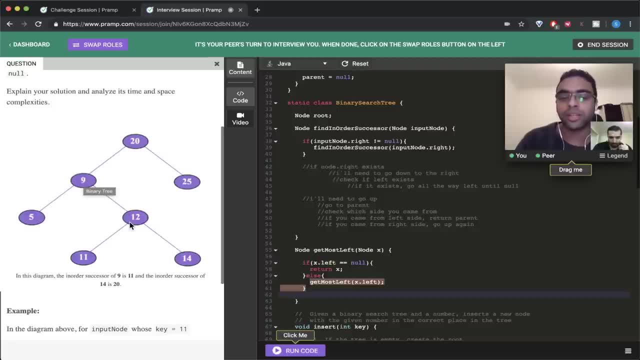 No, because it's equal 11.. Right, So you will go here and I trade again with 11.. So, and when you get, you got your 11. 11 dot left equal, equal null. Yeah, Okay, cool. 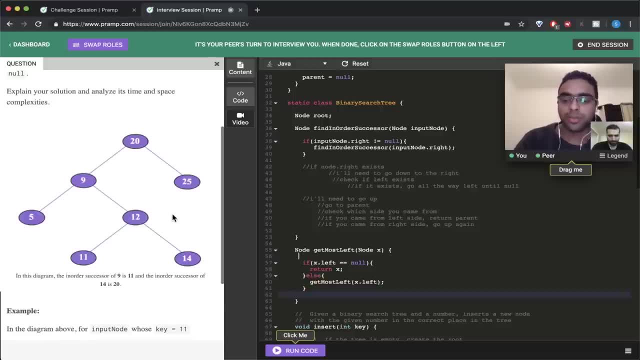 It's all right, It's working, Yeah, Cool, So we will done with this method, Right, Yeah, So here we need to do something like that, Right, Right, Okay, Yeah, That makes sense, Cause you're going to go to the right and then you're going to keep going to the left. 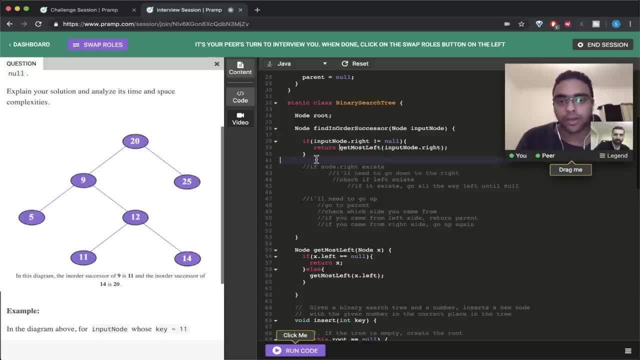 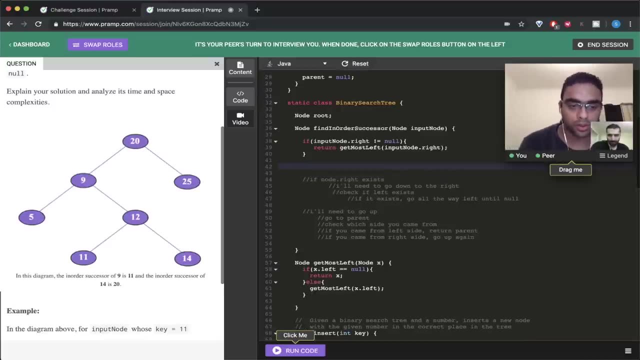 And here you need to return that, Right, Right, Okay. So I think that covers the first case. Yeah, Uh, let's go to the second one. Okay, So, um, so, yeah. so we said we need to go up now, so we'll say, um, maybe we'll have. 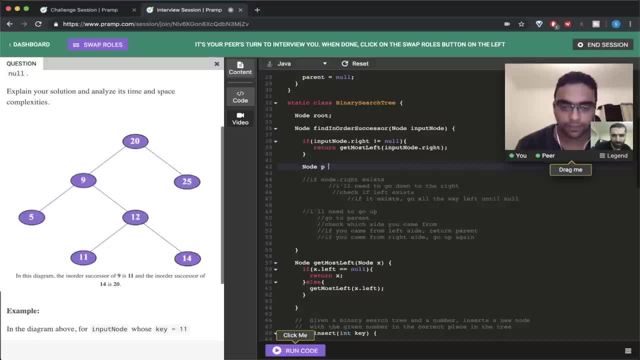 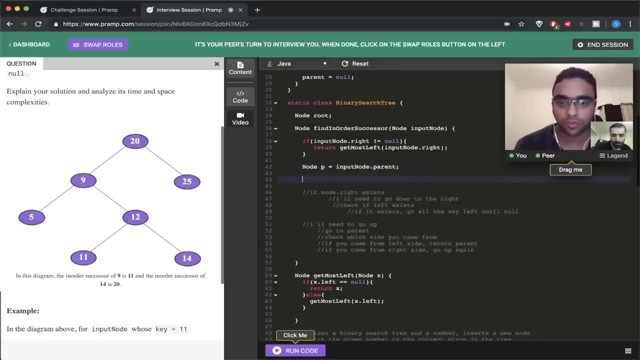 another pointer: Terrible, It's okay, Apparent, Um so So I guess. so right now we're kind of doing it the iterative way. Yeah, Okay, So yeah, let's just do it like that then, since 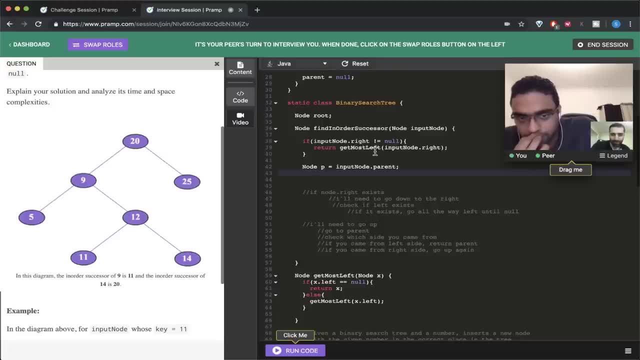 Okay, Okay. So if we have, if right does not equal null, we'll just go to the right and then go all the way to the left. Yeah, I think, I think we can call it in a more make sense. So we have parent right. 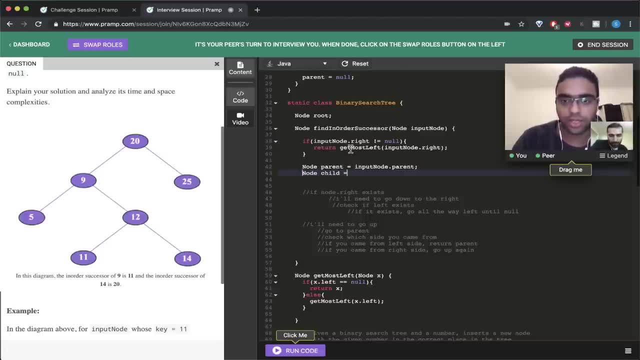 Yeah, And we have here some node- we can call it child- which is the current node, Right Right, Which is the input node right now. So we have child and we have parent. What we need to do, we need, we are sure now we need to go up right. 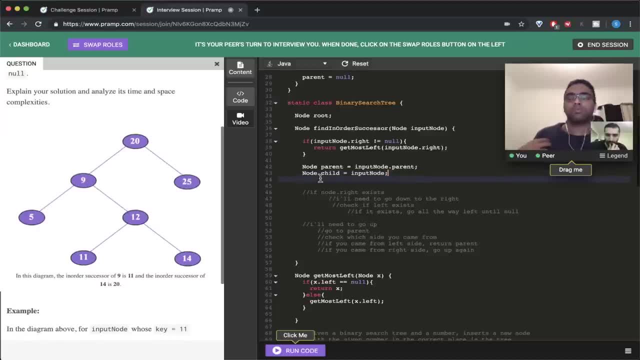 Right, So we need to do it iterative way, which is we need to do some while loop or something like that, but you need to define which condition. you need to stop iterating, right, Yeah, What do you think? So so this condition is: if parent dot left equals child. 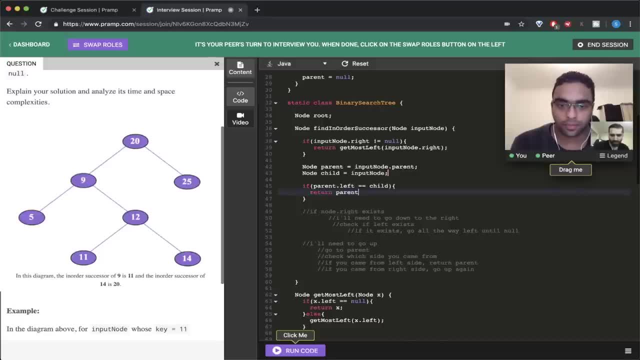 And then you want to return parent, or then you want to return yeah, parent. So what we need to do now, we need to reverse this condition and put it inside while loop. right, Um, yeah Cause, yeah Cause if the parent yeah. 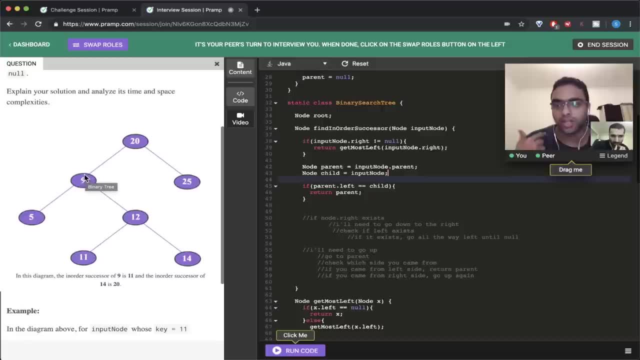 Cause, if this isn't true, then I need, I need to go up, right, We need to go up again, Exactly, Exactly. So if we change this one to be while and we do something like that, right, Just reversing what you said. 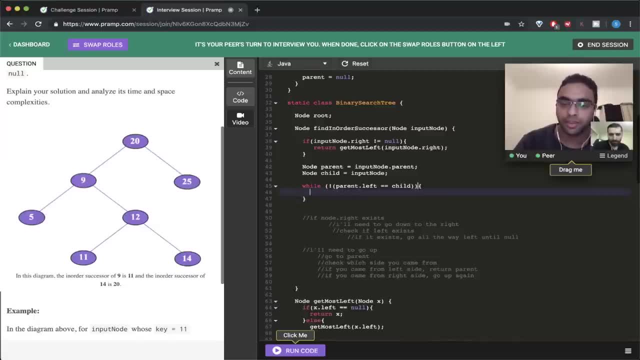 Yeah, Then you go. if I'm not going from the lift so I need to go up right. Your parent equals, So we can. we can just remove this part and instead of lift, we can do it A right. 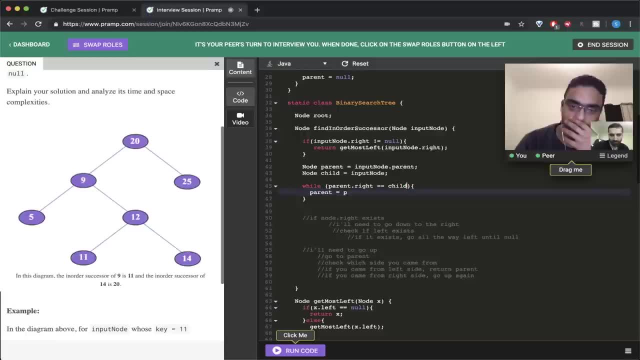 Exactly. Yeah Well, it equals, right. Then parent equals parent, dot parent Exactly. And for the child, you need to set First right And then right, Yeah, Child equals parent Exactly. And you need to just cover one extra check which you mentioned before. 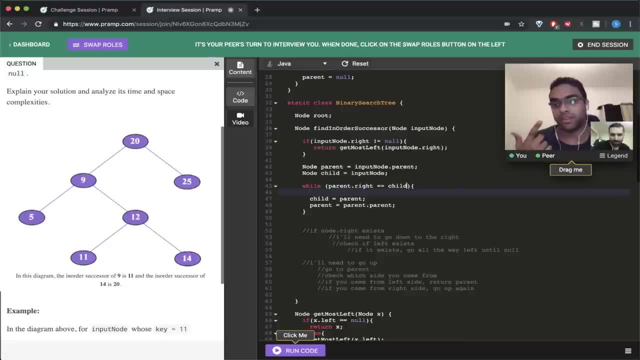 Yeah, If it equals. if it doesn't exist, Yeah Right. So we'll say: let me think where we need to put it for a sec. Okay, Yeah, I think we could just put it here: If parent dot, parent equals no. 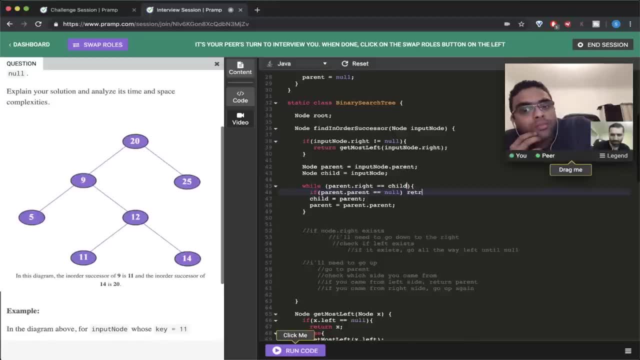 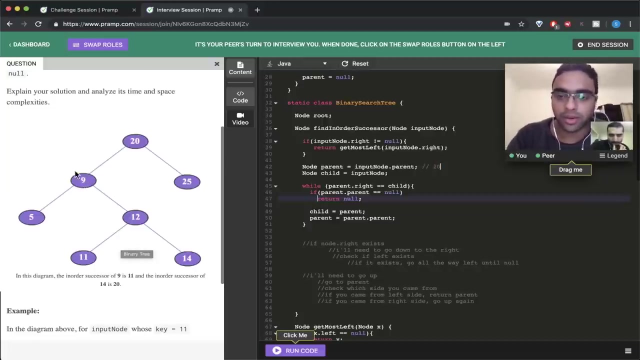 Then we're just returning. No, Think. think about the position for the condition again: If I give you, let us make some debugging. Okay, If I give you nine. so here's: the parent will be 20, right, The parent will be 20.. 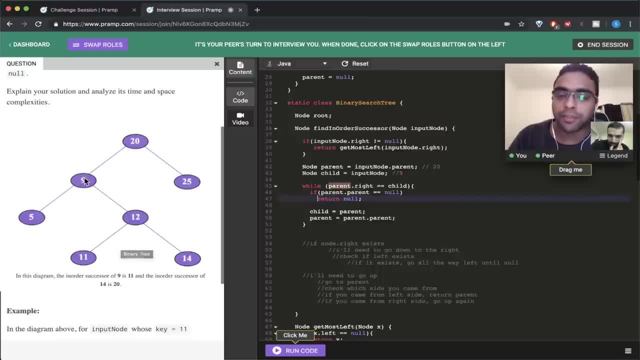 Yeah, And the child will be nine. I will check If the parent to try which is 12,, sorry, which is 20, to try 25 child. No, So I will. I will go inside this for loop: parent to parent: equal, equal null. 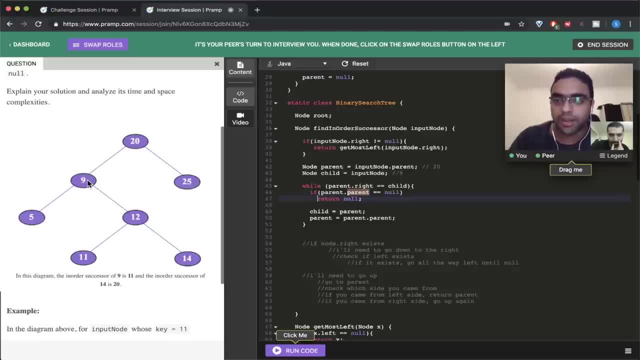 Right, Because the 20, the parent for 20 is not right. Um, so yeah, while parent thought right, Yeah, Wait. So parent the trite, equal, equal child. So parent is 20.. Yeah, Parent thought right. 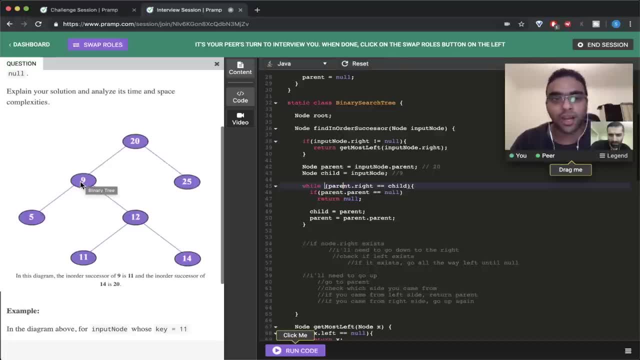 It doesn't equal child. Yeah, Oh, okay, That's makes sense, Right, So hold on. Um. so, while parent, right, Equals child. Um, sorry, someone's at the door, I think. um, so, yeah, so, so, yeah, so input. 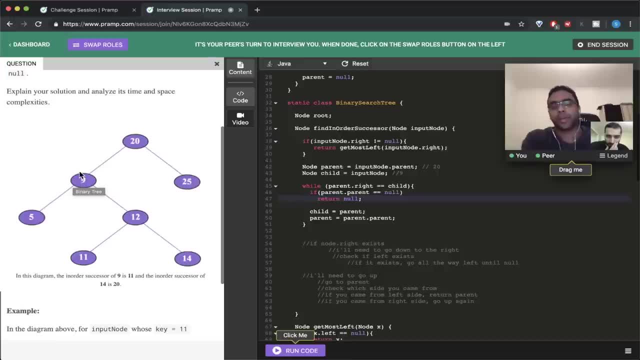 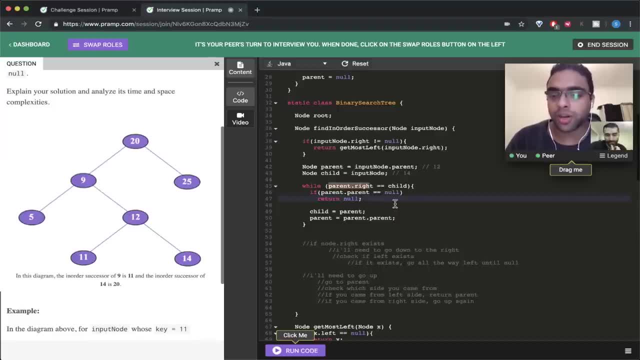 Okay, So we'll start from here. is parent to trite, which is 12 to trite, equal, equal, 14.. Excuse me, Actually, can you give me one second? Someone's at the door. Okay, Literally one minute. 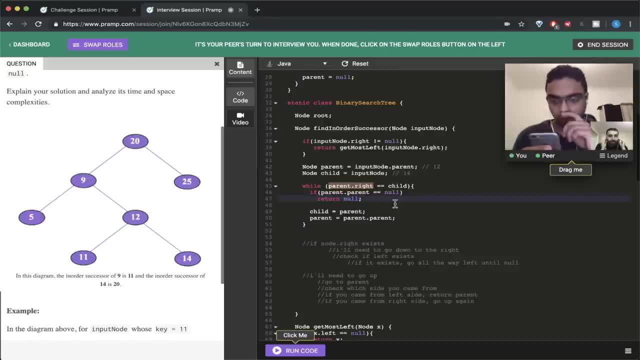 Sorry about that. Okay, All right, Sorry about that. No, no, no, It's okay, man. So the parent now was 12. Okay, Yeah, And the the child is 14. Okay, Why is it for? oh, so yeah. 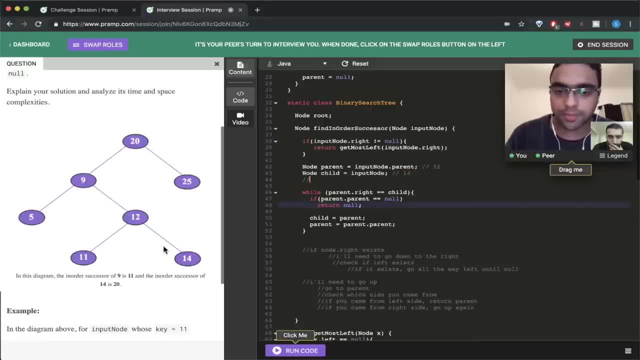 Okay, Yeah, It's child 14, parent. Yeah, And the parents. Well, so I'm expecting from you to return 20 for me. Okay, That's what I'm expecting. So we will start debugging the parent dot trite, which is 12 dot trite, equal, equal. 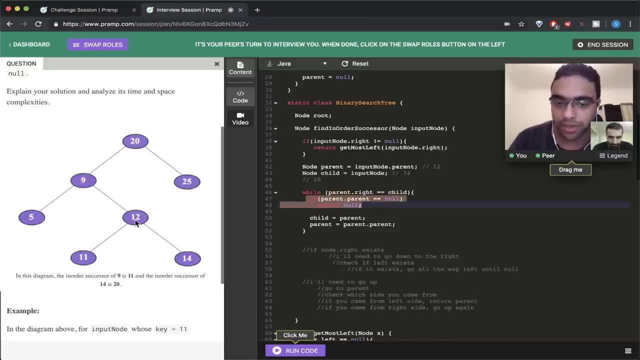 child equal 14 years. That's true, True. So I will. I will come here. if parent to parent equal equal null, No, because it's. it's equal to nine. So I will continue. The child will be 12 and now the parent will be nine. 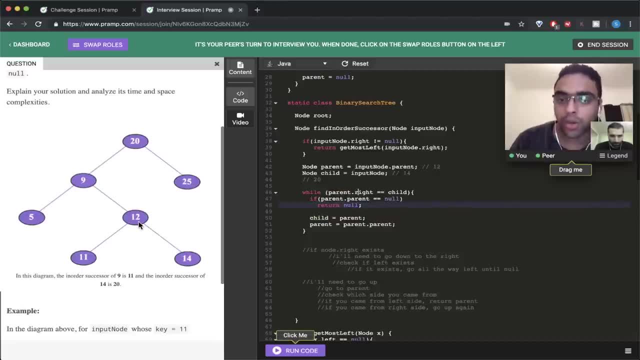 Right, Right, I will continue again. If nine Dot trite: equal equal child: Yes, That's true, So I will come here. If parent dot parent which is 20, equal equal null. No, So I will continue. 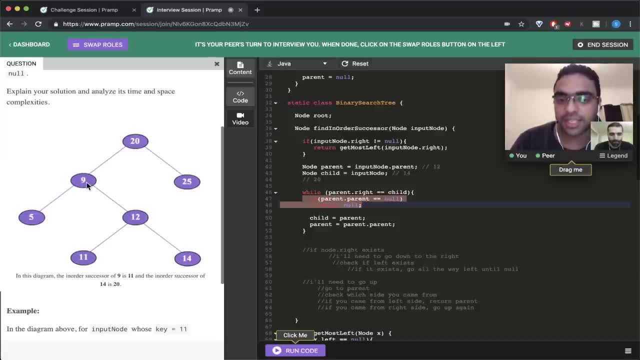 The child will be nine, Yeah, exactly, And the parent will be 20,, 20.. Yeah, And I will come back If the parent trite, which is 25, equal, equal child, which is nine. No, So I will come here and I will return the parent. 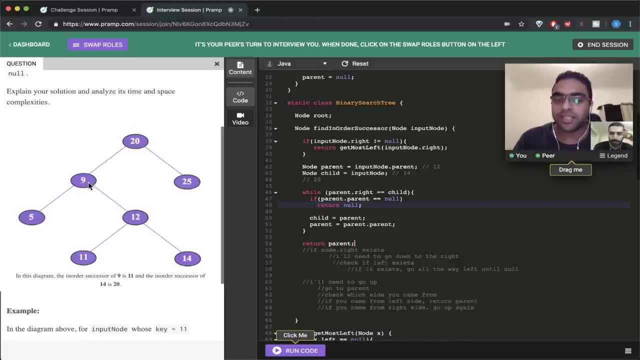 Right, Right. So that's working, but I think there's some Case It can be not working. Let me think how we can, how we can break that. So you see a. do you see a particular case that wouldn't work? 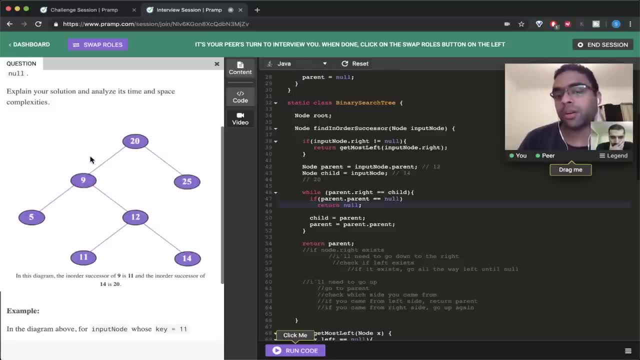 Yeah, I see a one. If I give you the input node, it's already null, Okay, Okay, Which is I gave you already And I'll input invalid input. Okay, What do you mean? Like like a node that's not in the tree? 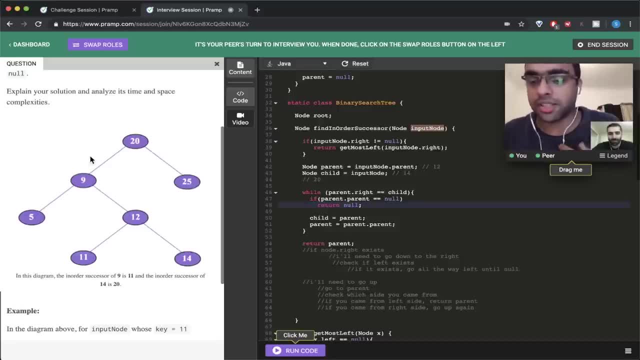 No, no, no, The node is not itself, is not? it's not an invalid input, Right Yeah? So if you will do it here, which is null dot trite, it would be so an exception, right Yeah. 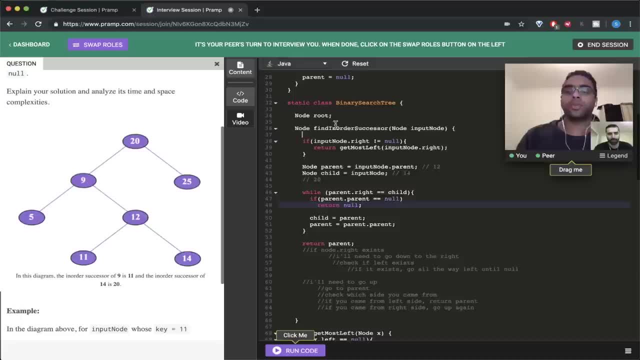 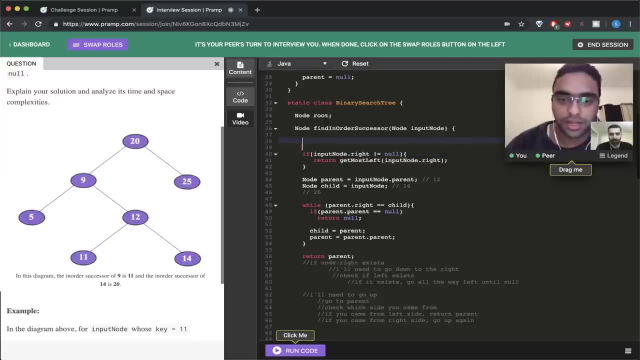 Can we just do a check? Yeah, exactly. So at the beginning we need to check if the input node not equal null or equal equal null. we just need to return anything Right. We'll just return null, Right, Exactly. 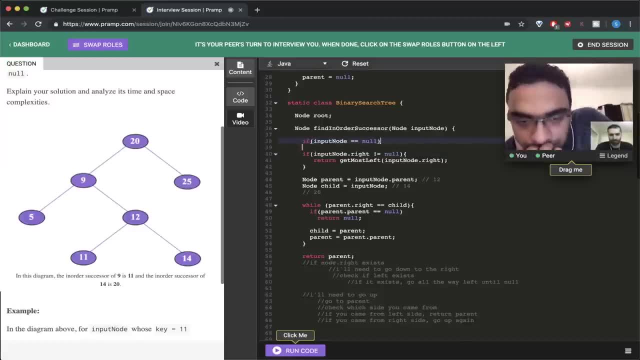 And I'm thinking about different case- What if? um, I think we should cover all the cases. Yeah, Yeah, I think that's working fine. Yeah, But let me think about if we can break it. Okay, Yeah, Let me think. 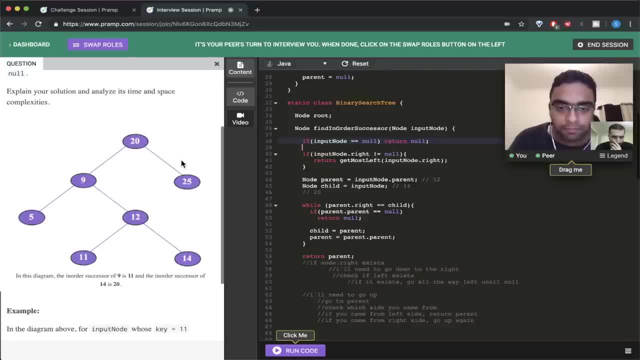 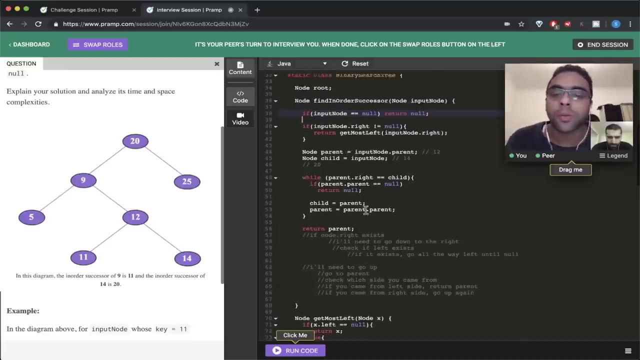 Um, so you said it's true, right, And I think it will help. Thank you, Yeah, I think it's going to work. Go ahead And then let's see what else it can be. Let's check Um. 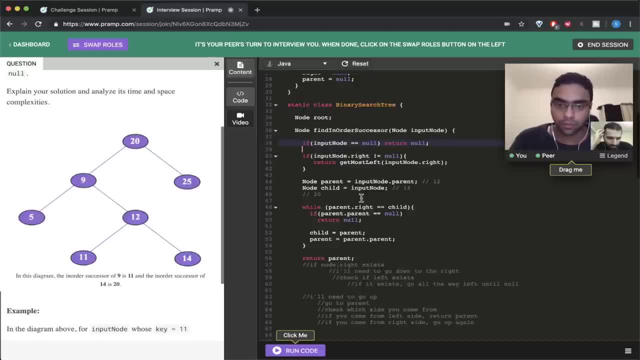 So let's see, since it's over a couple of pages. Yeah, Well, uh, i think it should be log of n. okay, why log of n? um? well, just from looking at it, i know when we're going up the tree we're only looking at the. 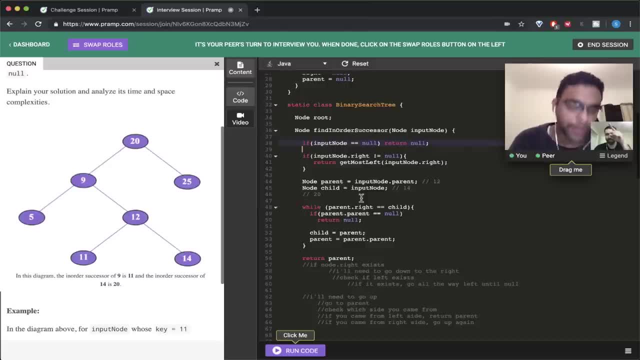 the nodes that are on that particular path. and, okay, like if we want to trace it the other way around. we know that we're only checking half of the tree each time. and what is the height of the tree? um, well, i guess, if the height of the tree is n. 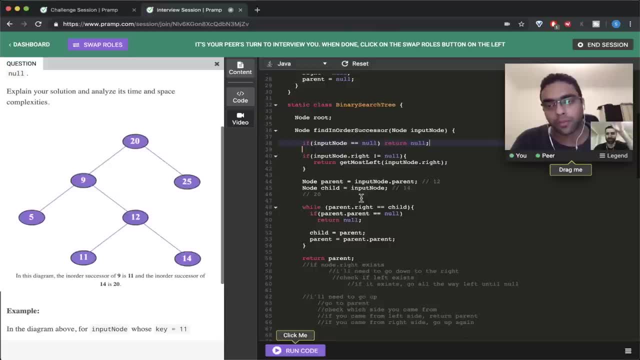 say we have, say we just have like one, say it just goes one way and everyone only has like a right or a left, then yeah, then you would be looking at every so, yeah, so, yeah. so in in the best case scenario, the height for the pioneering search tree is log n right, because 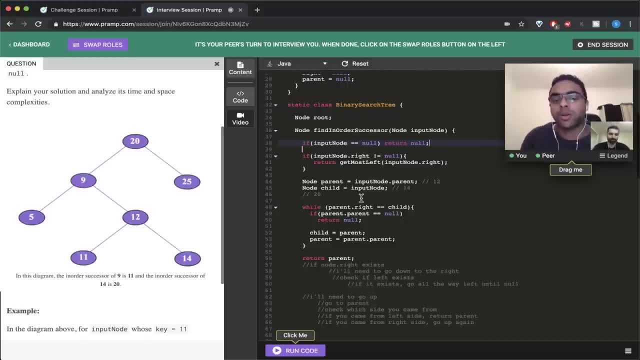 it's a pioneering search tree. but in the worst case scenario, which is we only have nodes in a only one way, which is only right, only left, we can have a chain which is called a chain problem, and it will be a linear right, right. so the time complexity in the worst case scenario will be: 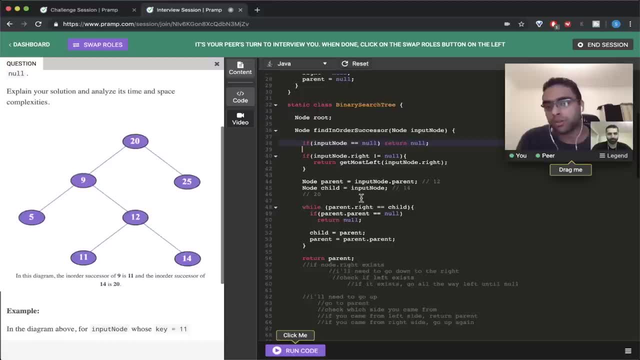 order n, but in amortized log time or the average running time, it will be order log n, as you mentioned. and what's the space complexity um? the space complexity um will be um, since we're not calling it recursively um, it should just be constant space. yeah, cool i. 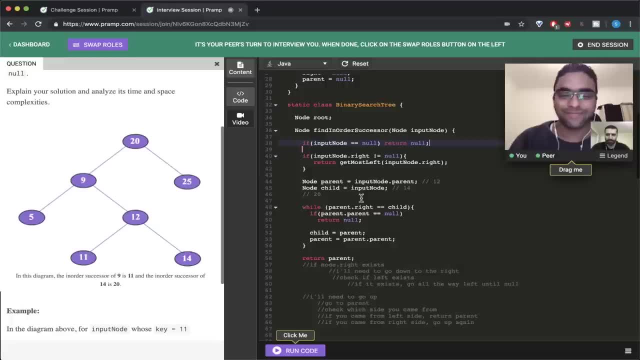 agree with you. yeah, you're done man well actually when we're doing get most left, yeah, then if we have, like you said, only if everything is to the left, then yeah, i agree with you. but in the worst case scenario you are not iterating through all of the nodes because 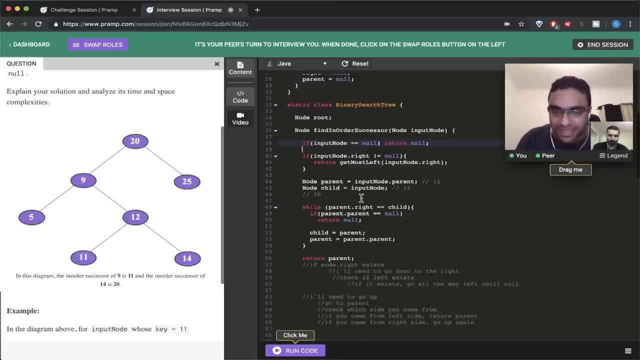 you will. to get this point you have, you need to have at least one right, node, right, um, yeah, yes, okay, so if you have one right, exactly, exactly so, it would be another and minus one, you know? yeah, you can discuss this with the interviewer. both of them are valid, but i think, for me, constant. 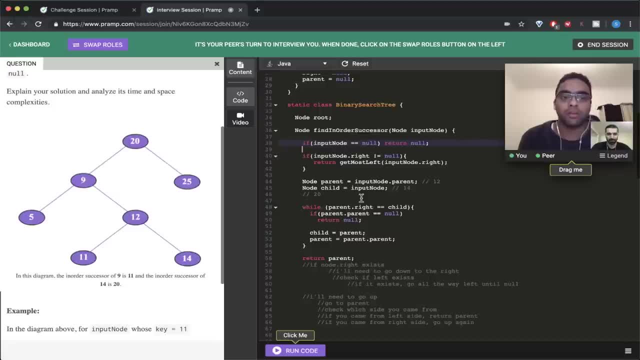 it will be a satisfied answer. and this is what i have in my, in my model, and we could also- we could write- get most left as the iterative approach where we just use a pointer and then it would be no space. but you can do that, but in my case i would 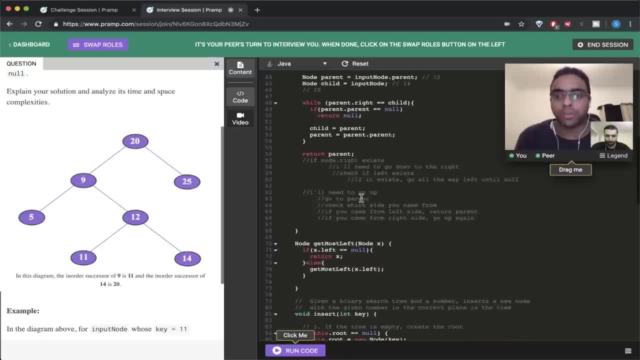 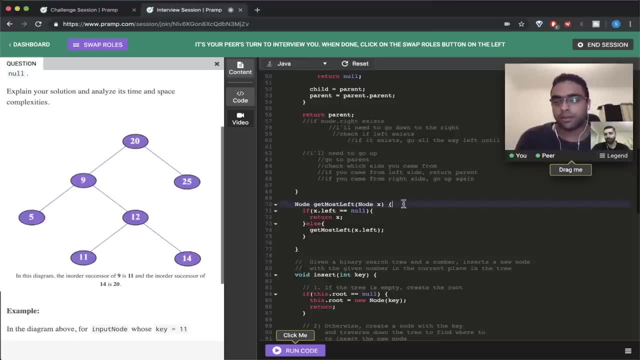 because if you want to do that, you need, you need extra space. you need because you need to keep track with the most left node, right, um, yeah, i mean you would have the extra, you'd have the pointer. so, oh yeah, just, just, just, you need, you need extra memory inside each node. you need because 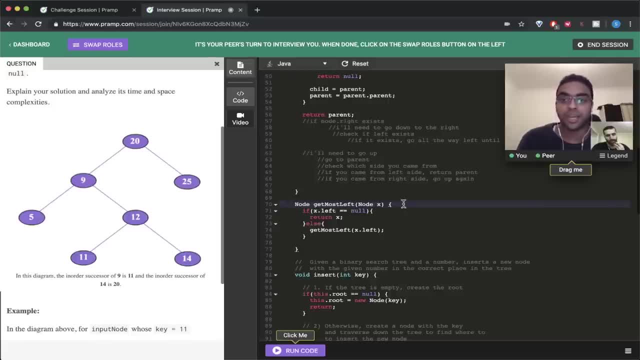 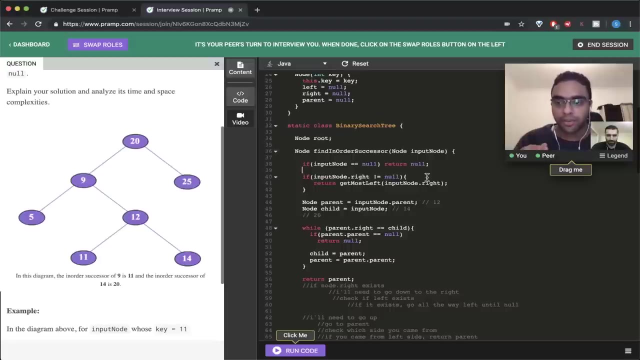 you want each node to point to the most left node in the same path, but you can't do that because you will break another thing if you want to keep a pointer inside the node itself which can point to the most left node inside the same path every time you insert a new node. 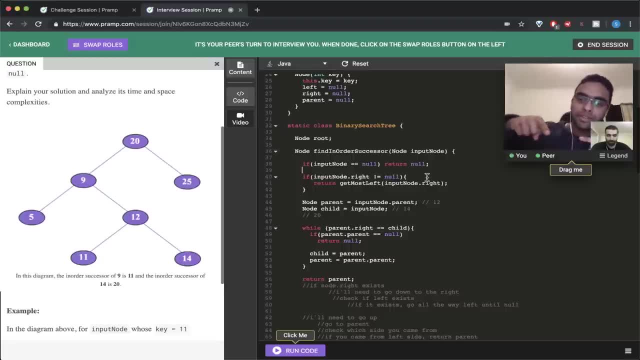 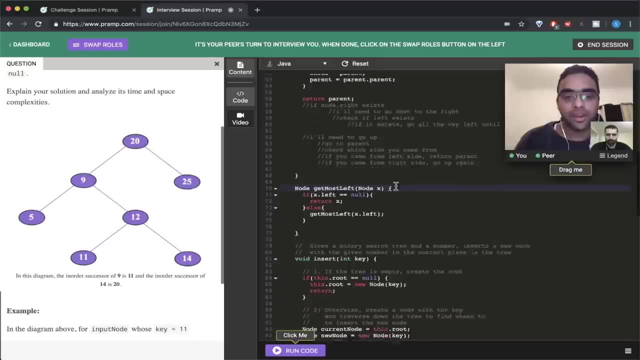 in the pointer search tree, you need to go in the full path and update all of them again, right? so let me think, if we back to the same question here in in in 12- well, i'm just thinking um in line 70 on this, this function. here can we just have a pointer that just goes all the way to the 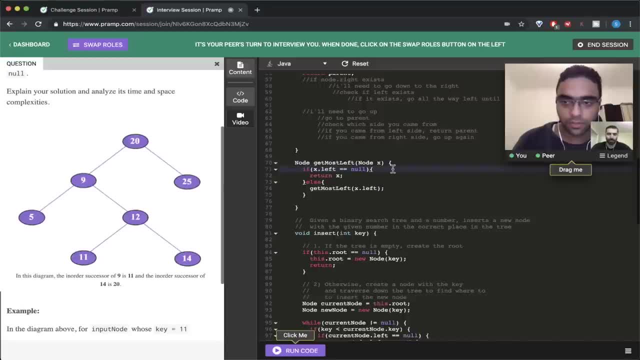 left until we hit a node. yeah, there's a problem because if you insert a new node which will change the some order for some of the node, you need to reorder the same right. you need to reorder, reorder this pointer in all the node right and that will break the condition that we can insert. 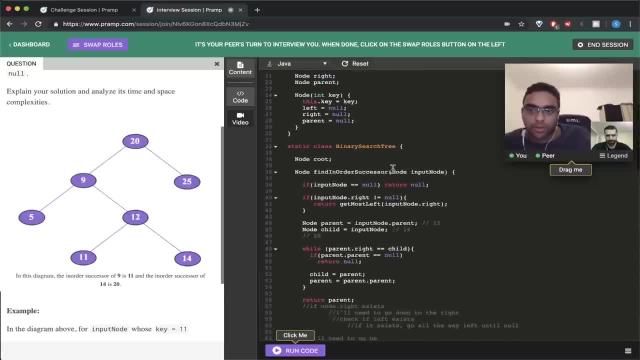 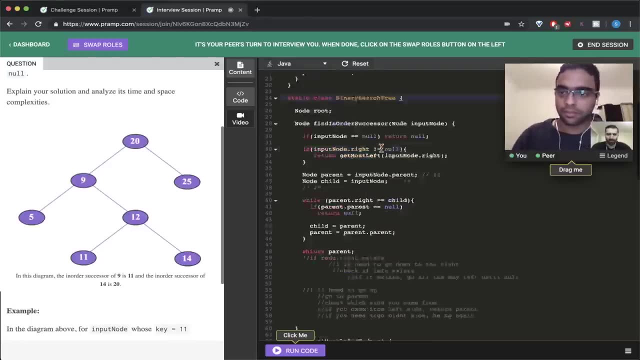 in the pioneer search tree in log time. right, so it will violate another another conditions, but okay, okay, cool, all right. uh, is there any way we can run it or are we just gonna? there's no test cases. are there? i think i can run it. it's running now. 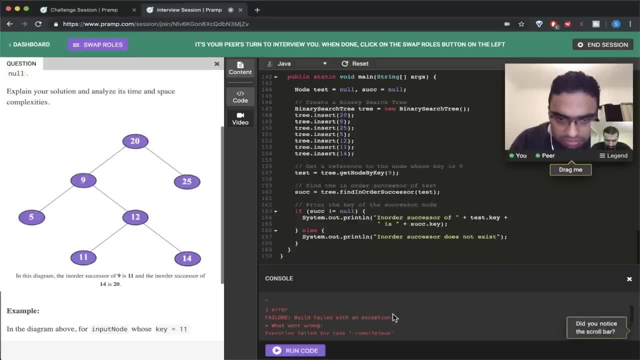 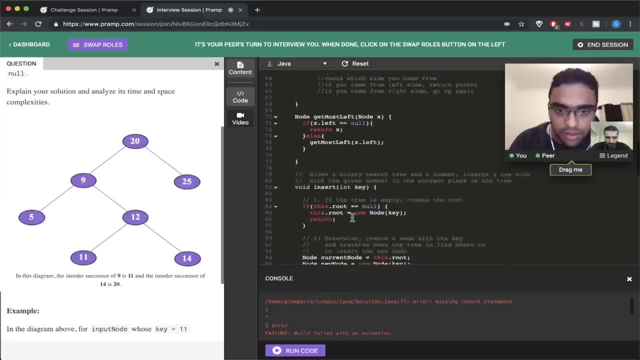 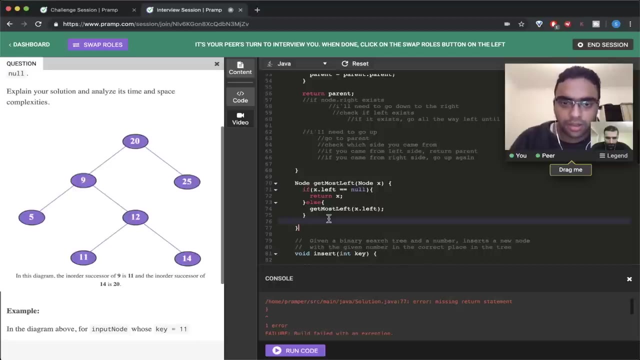 okay, um, you have some missing return datum in 77. let me check that 77. well, why not? okay. so if we just get rid of the else, yeah, or we can just get rid of the else, yeah, okay, i think that could- and return, and so you have expecting a line 73, what we have. 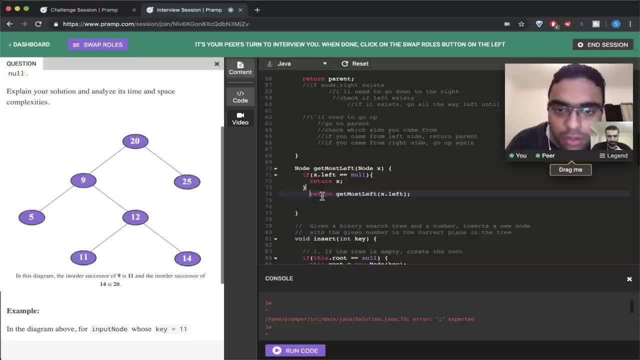 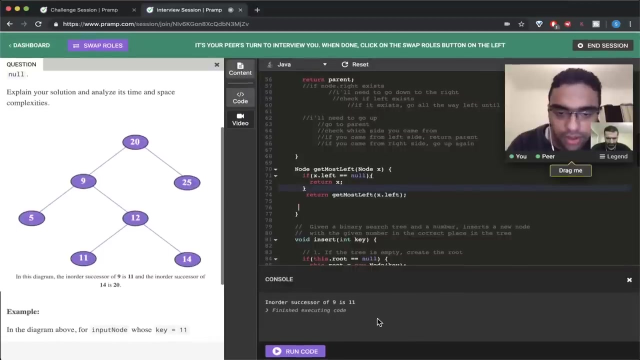 i don't, uh. so, error, not a statement. where is the e? i don't find the e. yeah, i don't know. uh, uh, maybe let's try it again. maybe, uh, we were both typing and maybe it got messed up. okay, yeah, it's running now and it's working. okay, cool, cool. 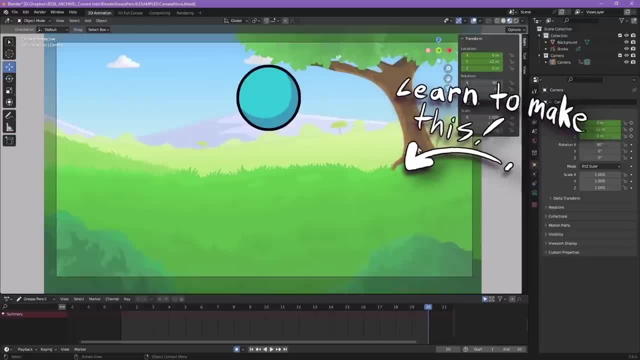 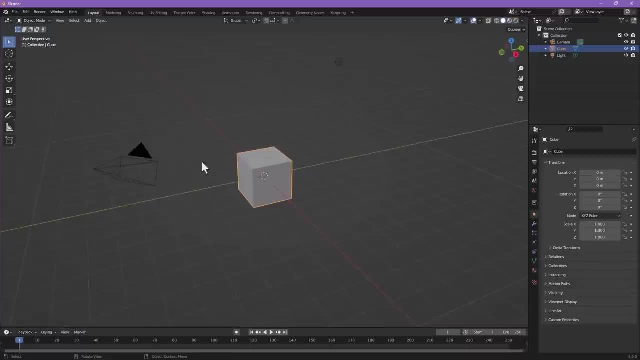 In this tutorial we're going to go over how to animate in 2D in Blender. even if you've never touched a 3D program before, Blender may seem like a complicated program because of its 3D nature, but I guarantee you by the end of this you'll be animating in it. 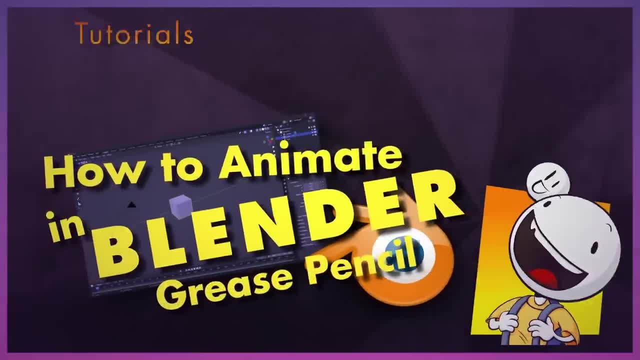 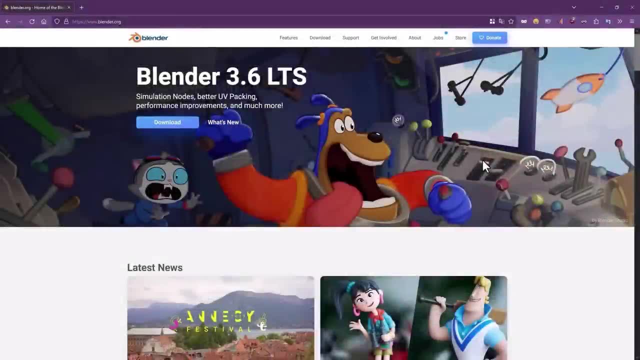 in no time. So let's get started. If you don't have Blender already, you want to go to blenderorg and click the big download button to download Blender. the version that we're using in this tutorial is version 3.6.. So once you have that downloaded and 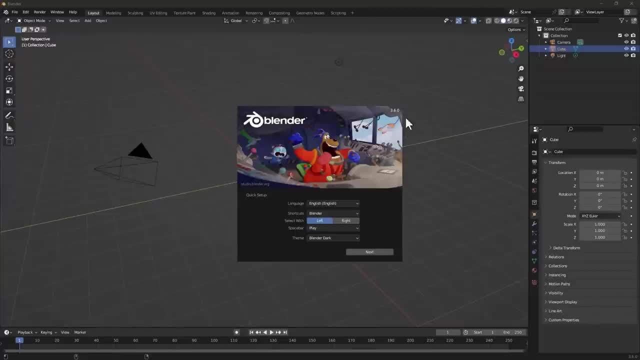 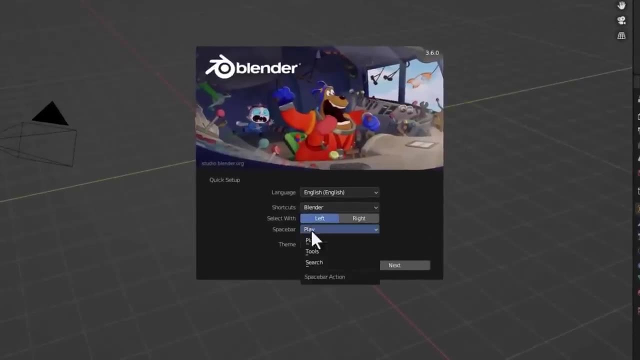 installed, you'll be greeted with this welcome screen. So I recommend keeping all these settings to default, except for the spacebar option. The spacebar: personally, I like to have it set to search, and that's useful because there's so many things in Blender that it can be hard to remember. 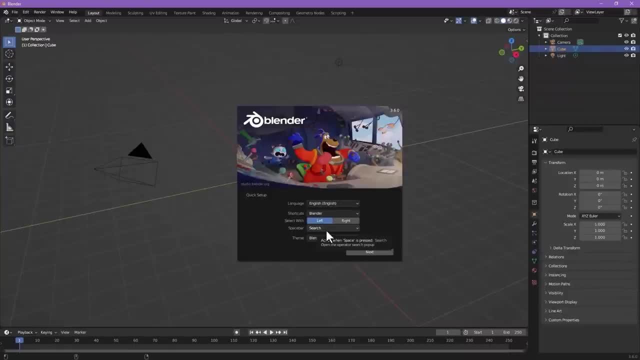 where things are. So instead I could just press spacebar and search for what I'm looking for really quickly. So I recommend that. So once you have that set up, click next. So that's it for this tutorial. If you want to learn more about Blender. 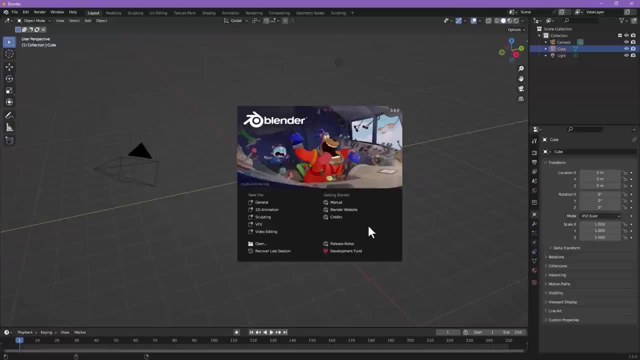 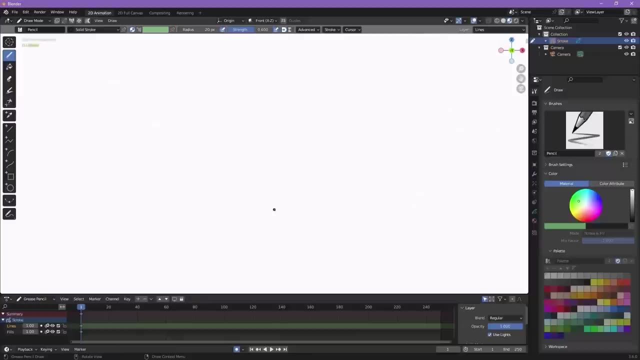 that setup window only happens once. Usually when you start Blender you'll see this welcome screen right here. So to make a 2D animation, we simply click 2D animation in this welcome screen and it'll set up a new project that's ready to animate in 2D. If, for some reason, you don't see,